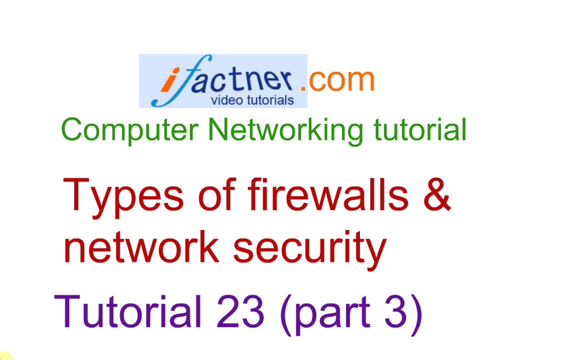 What's up, guys? rfechnercom is here and I welcome you to computer networking tutorial and we will continue our discussion on types of firewalls. So this is the part 3 of 3 part tutorial series on firewalls, and in part 1 I introduced you to the concept of firewall. 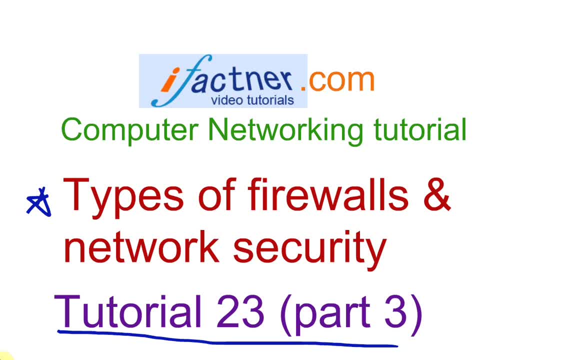 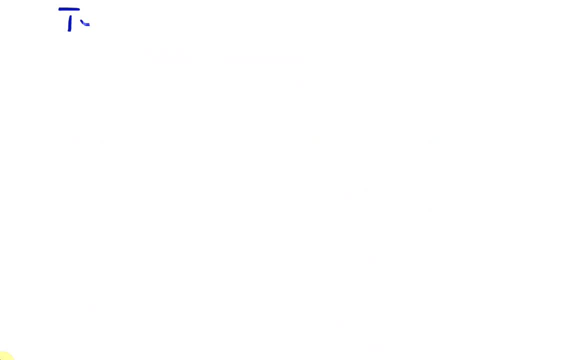 In the second part, we discussed about the generations of firewalls and in this part, we will be discussing about different types of firewalls that are available in the market. So, guys and girls, you would be happy to know that we have already discussed some types of the firewalls in the second tutorial, that is, the generations of the firewalls, and we 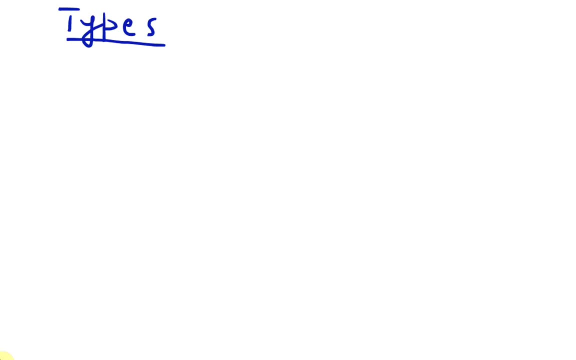 would be further discussing those types. So first type of the firewalls are called packet filters and we have already discussed that. there are two types of packet filters. Number one are the stateless packet filters that were introduced in 1980. And they only checked the authenticity of the packets. and the second type of the packet 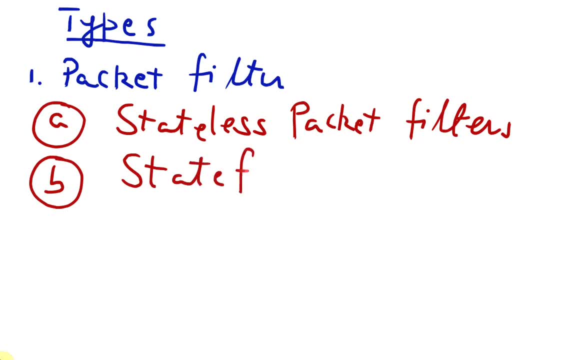 filters are the stateful packet filters and they check if the packet is a part of the existing communication or if it's the part of a new communication or if that packet is not a part of any communication And based on these three states, it can decide what to do based on the predefined rules. 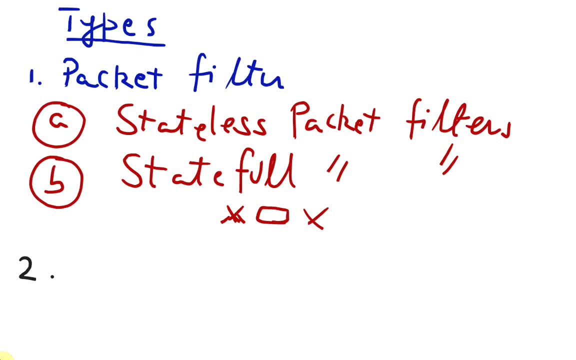 And the second type of the firewalls which we have already discussed in the generations of firewalls is called the application layer firewall. So application layer firewall mostly works in combination of packet filters, especially the stateful packet filters, and it works on the application layer of the firewalls. and 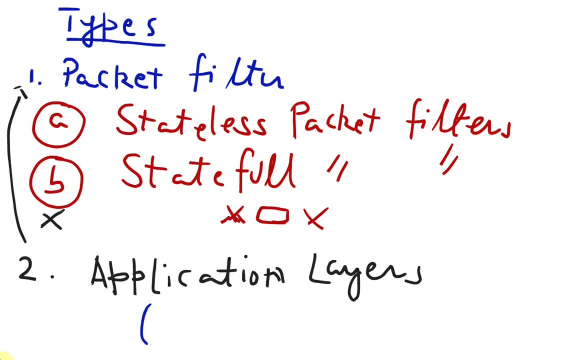 it can basically check the authenticity of the packets, the connection status and the ports or ports and the protocols of the packet. and if those ports and protocols are allowed, then application layers- filters- would allow the packet to either enter into our system or the network or to go out to the internet. 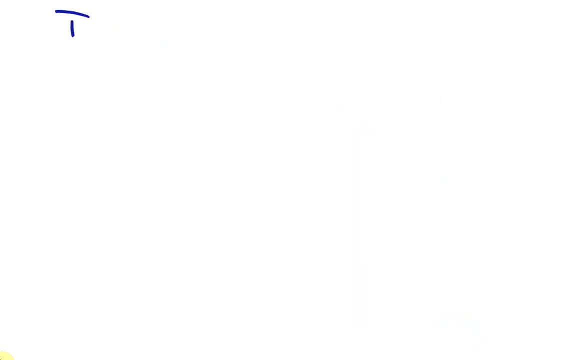 And the third type of the firewalls which we would be discussing today are called proxy servers or the proxy firewalls. And the fourth type which we would be discussing are called the NAT firewalls or Network Address Translation Firewalls. Some people say that there is another kind of firewall that is called the new generation. 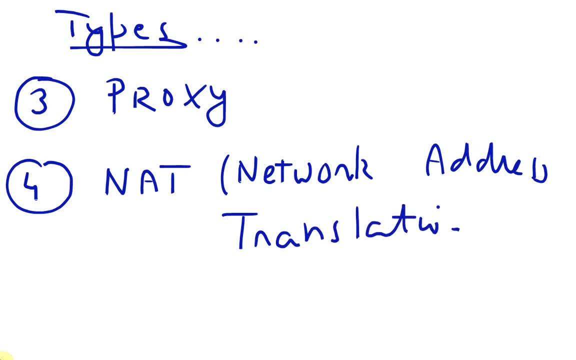 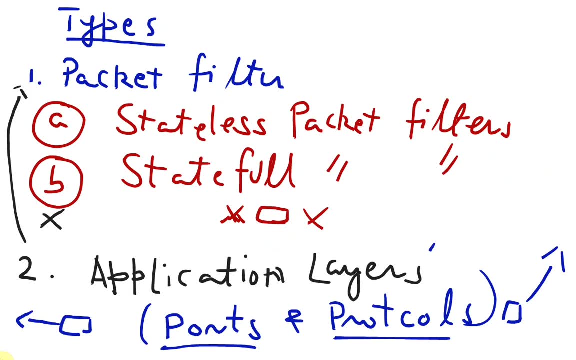 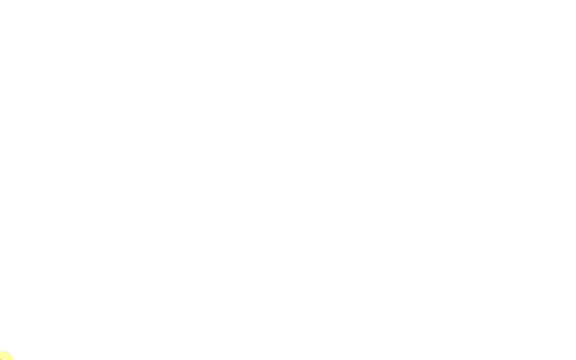 of the firewalls, but I would say that they are just the network address translation firewalls, The newer version of the application layer firewalls, and they do the deep packet inspection. So now let's discuss about proxies. So first let me tell you what is a proxy server. 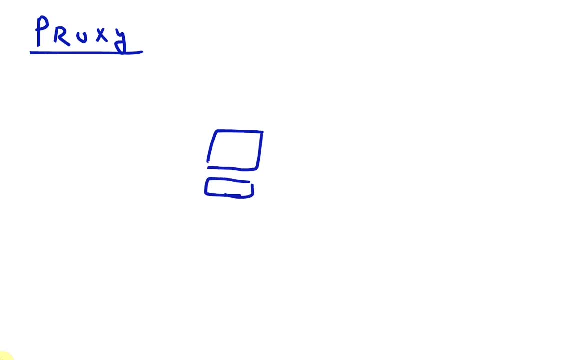 A proxy server. you can think of a proxy server as a server which sits between your local area network and the external network. So what is a proxy server? A proxy server is a server which sits between your local area network and the external network. 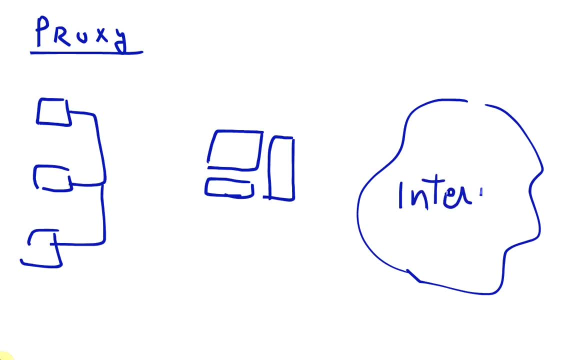 This server is a network, that is, the network of the internet, And all the communication is done via this proxy server. So you can think of it as a firewall, because in this proxy server we can allow the protocols that can be used for communication. 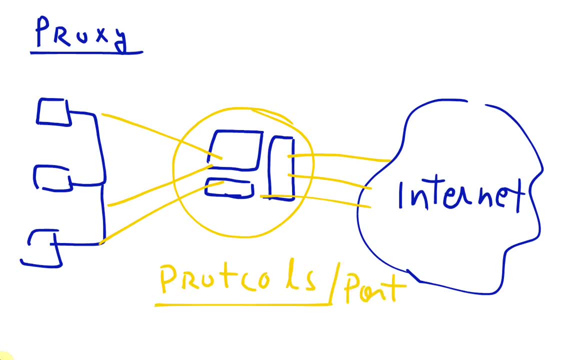 ports which are open and which are closed, and we can also define different set of rules. we can block the websites or different services of the internet based using the proxy servers, and the advantage of proxy server is that if we have got one internet connection and we would like to share it with all the 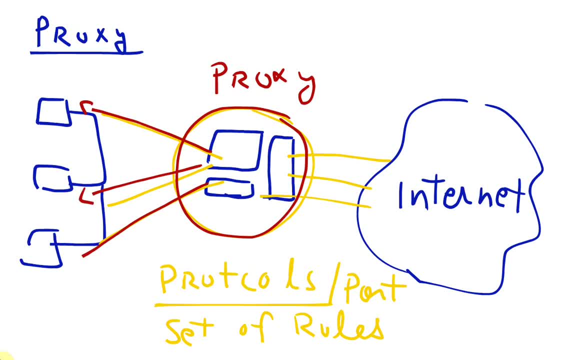 computers on our network, then we can use the proxy servers and the proxy server access and firewall, because it it is between our computers and the internet and it prevents the unauthorized packets or the unauthorized connection request not to go out or in the system. so these are called the third type of the firewalls that are the proxy server. 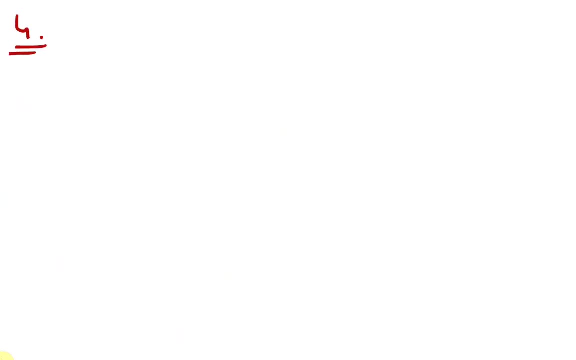 the fourth type of the firewalls are called network address translation or NAT firewalls and basically the network addresses, private network address system, or the table, was developed to facilitate the organization's which had a large number of PCs, so in an ideal case they would had to. 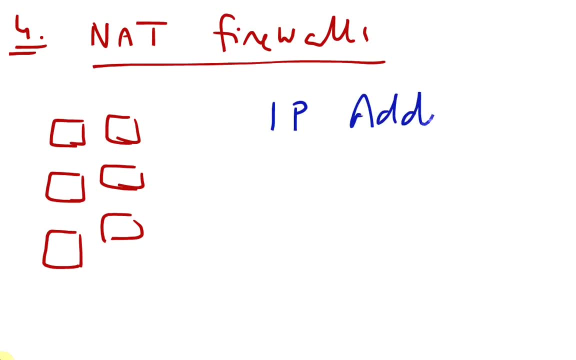 buy the public IP addresses, and that would cost a lot of money. therefore, our NAT system was developed, based on which they are the private addresses and the private address table, and there We have internal networkNS addresses for each of the pieces in the internal network, and then it has a public IP. it can also follow up with public IP addresses. so